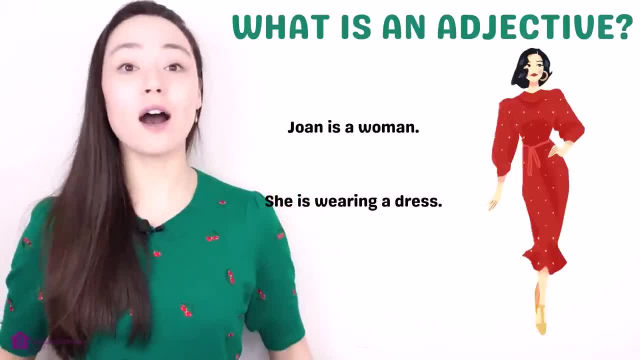 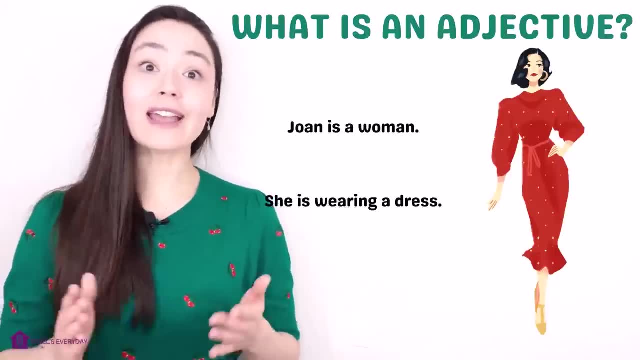 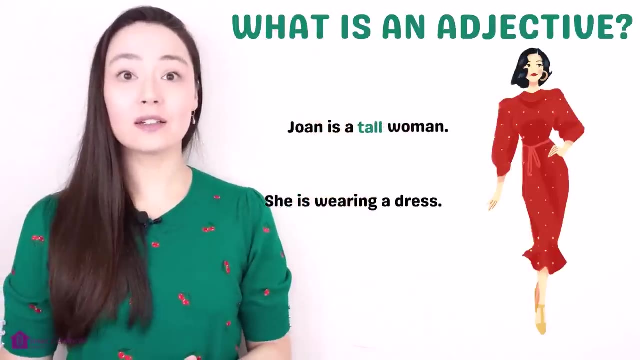 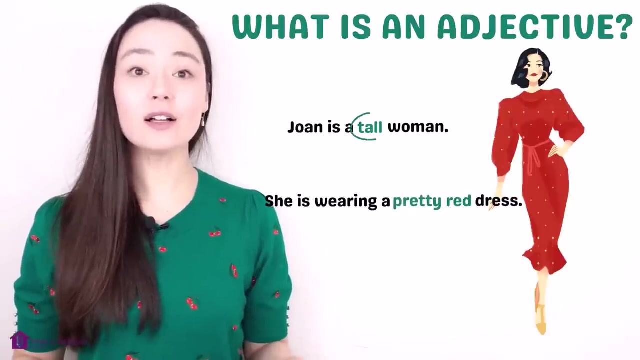 Joan is a woman, She is wearing a dress. How can I make these sentences more interesting? Well, I can add adjectives. Joan is a tall woman. She is wearing a pretty red dress. Tall, pretty red, those are my adjectives. 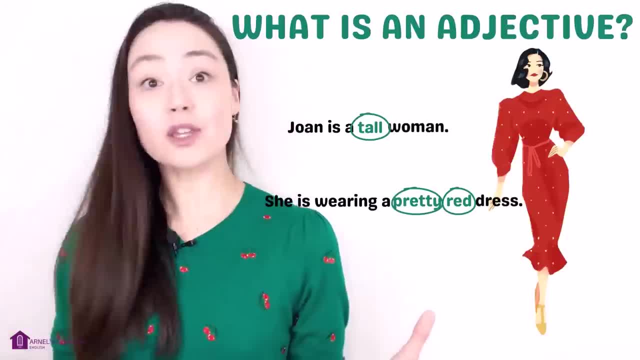 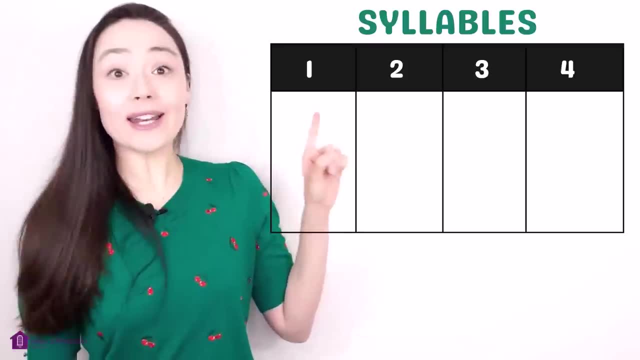 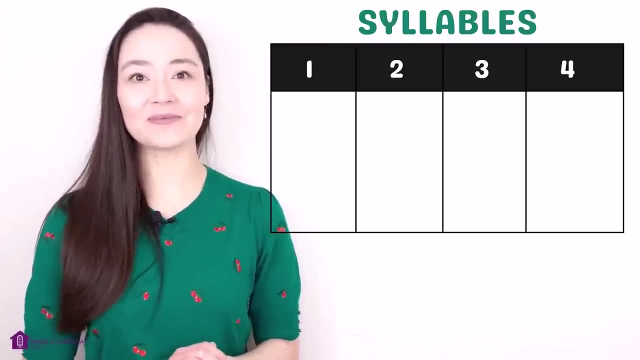 Look around your room, your classroom, Your office. What adjectives can you think of? What is a syllable? If you don't know what a syllable is, we can't continue with this lesson. One, two, three, four syllables. Fast. Fast has one syllable. 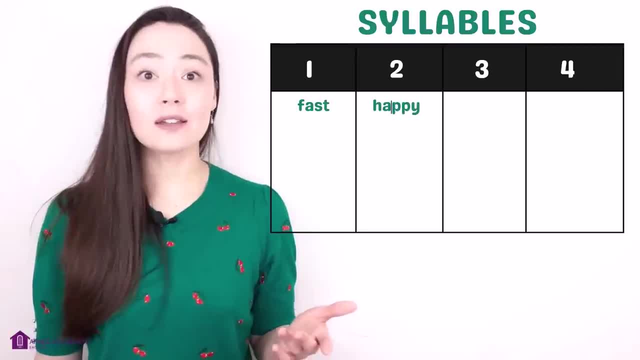 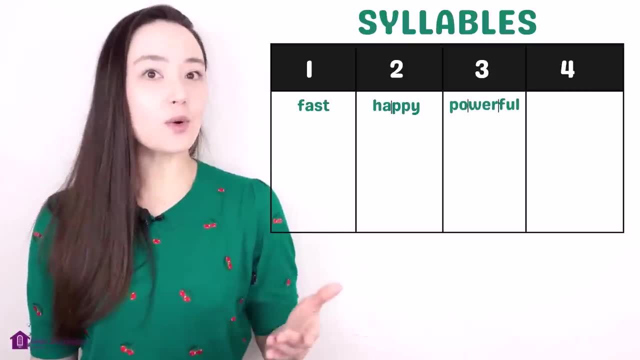 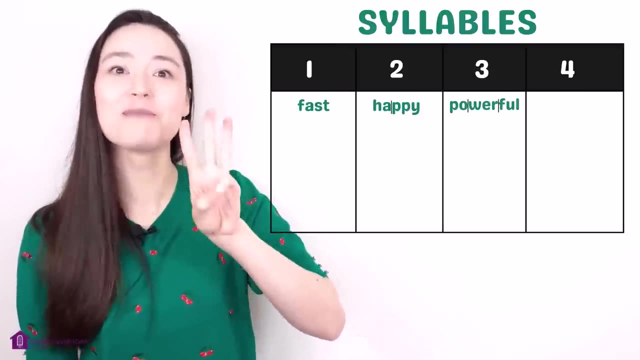 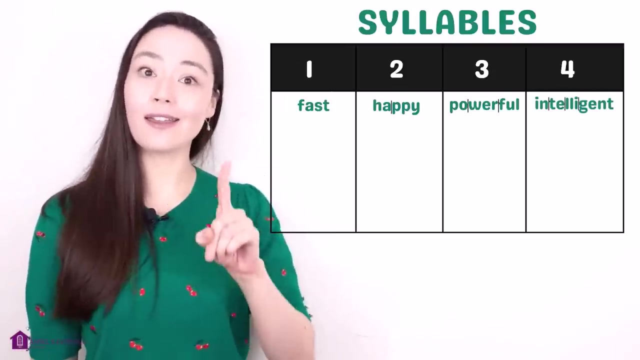 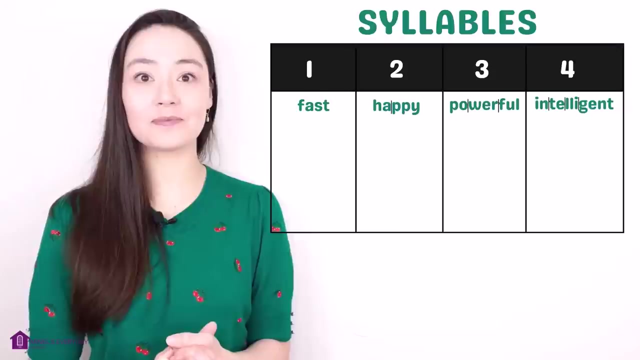 Mm Happy. Happy has two syllables. Ha-ppy Happy. Powerful, Powerful has three syllables. Pa-wer-ful, Three syllables. Powerful Intelligent, Intelligent has four syllables In-te-li-gent. You can see, a syllable is a brick in the pronunciation. 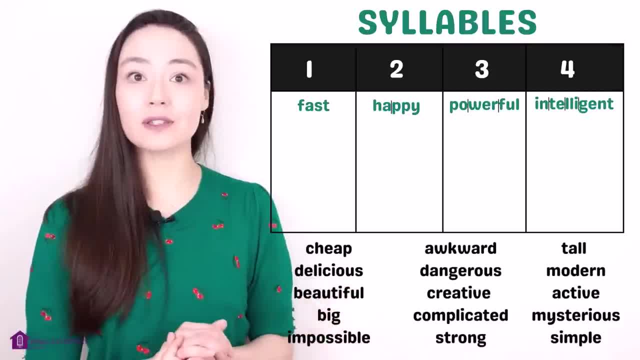 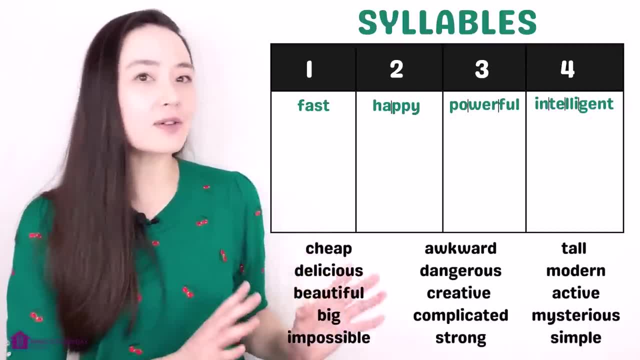 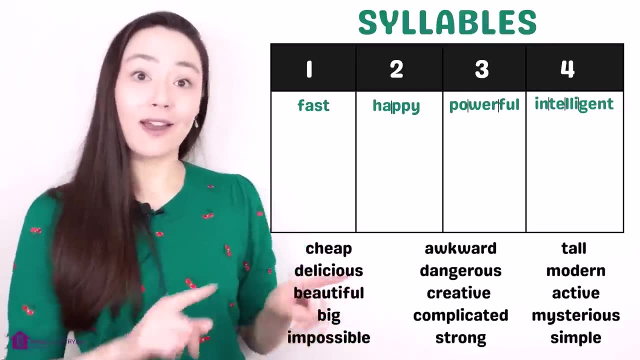 Here are 15 more adjectives In today's lesson. I just want to focus on the grammar so I'm not going to give you the definitions of these adjectives. Use your favorite dictionary or translator. Can you please put these adjectives into their correct? 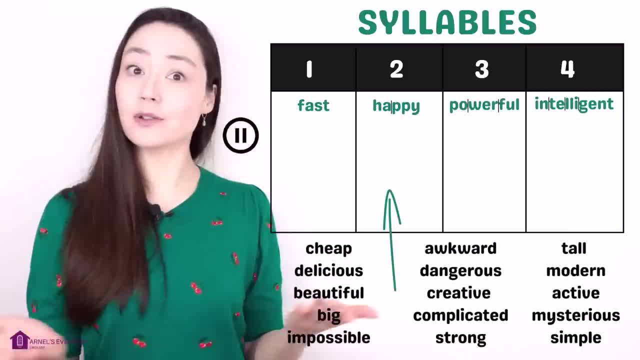 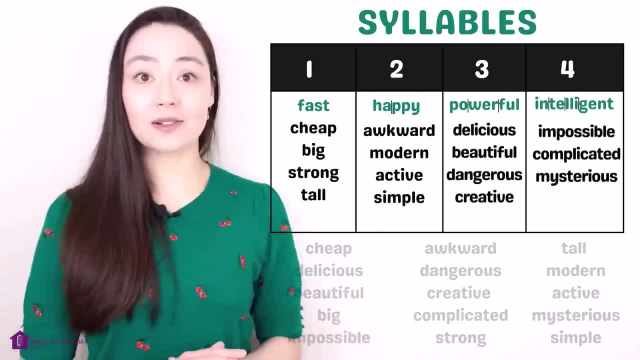 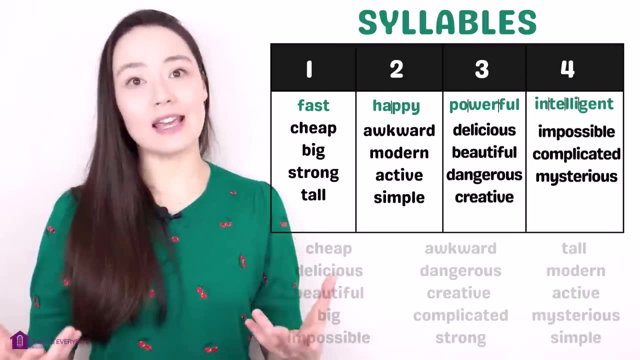 Correct Columns. Pause the video to do this. Here are the answers. Now that you know what syllables are, we can continue, And in English. yes, there are plenty of words with more than four syllables, but in today's 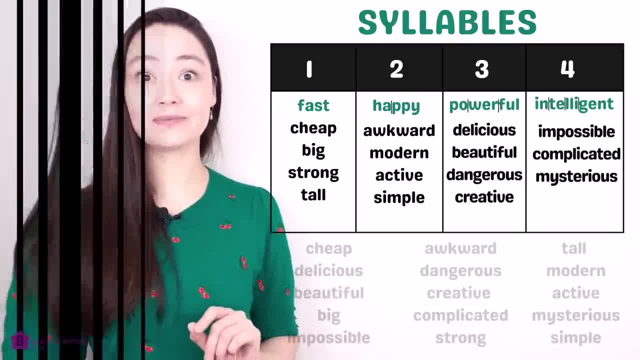 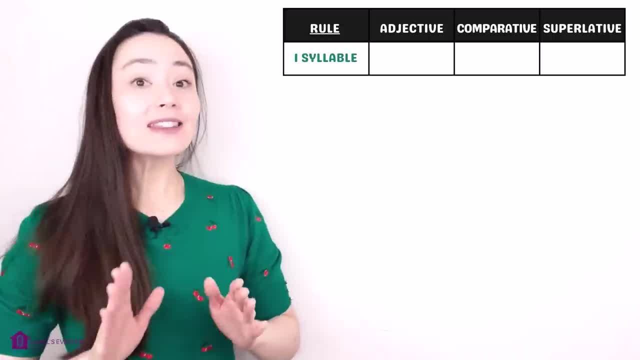 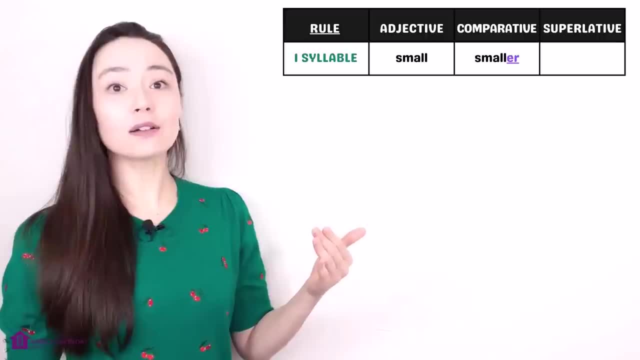 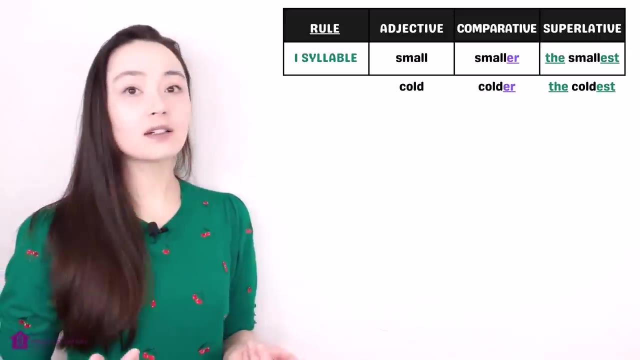 lesson. I think four is enough. I have a chart here. Adjectives, comparatives, superlatives. Let's start with adjectives with one syllable: Small, smaller the smallest. Cold, colder the coldest. Loud, louder the loudest. 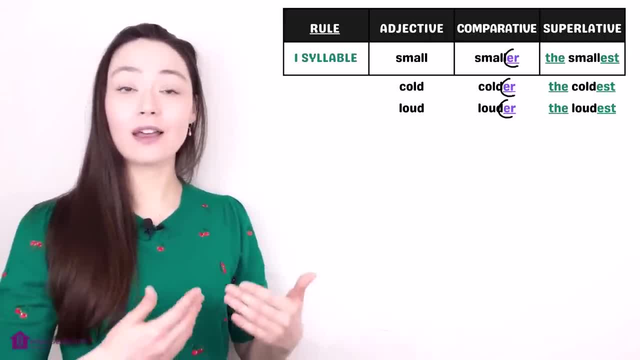 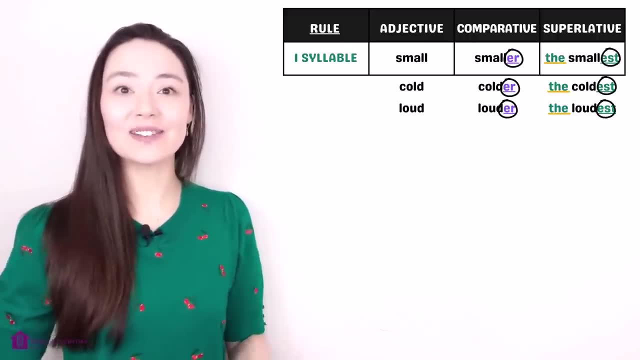 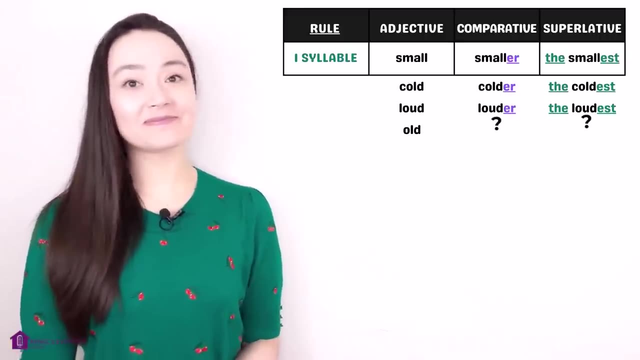 You can see, to form a comparative, I add forces And for the superlative, the plus E-S-T. Here's an adjective: old. What are the comparative and superlative forms? Right, Old, older, the oldest. 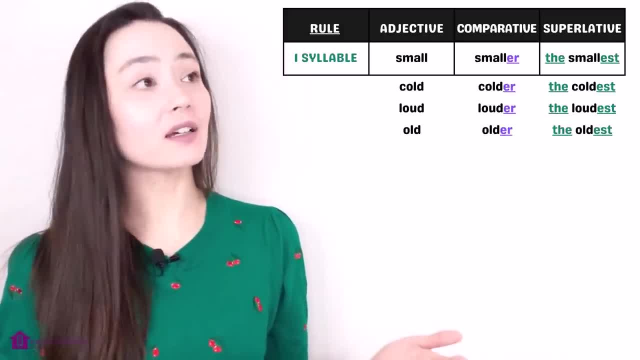 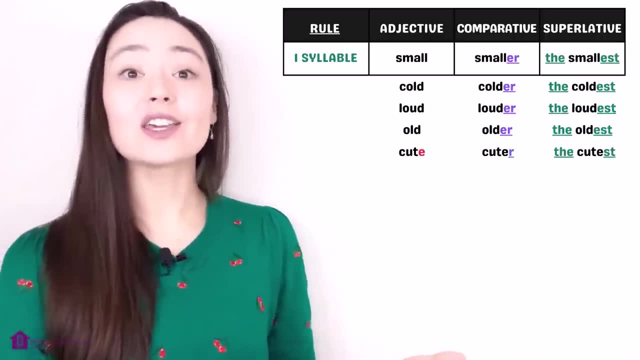 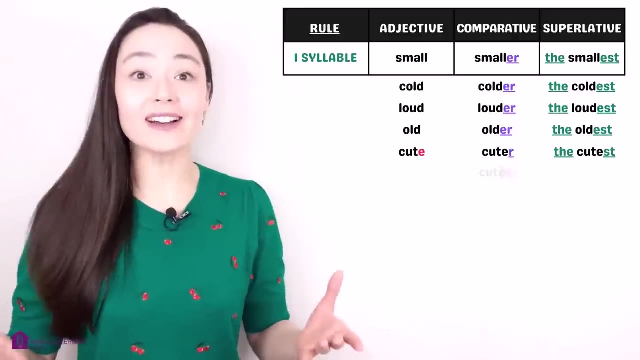 If your adjective already ends in E, like cute, we just add the R and S-T: Cuter, the cutest. We don't need to say or write cutie-er. Okay, the forms are clear, But when do we use a comparative? 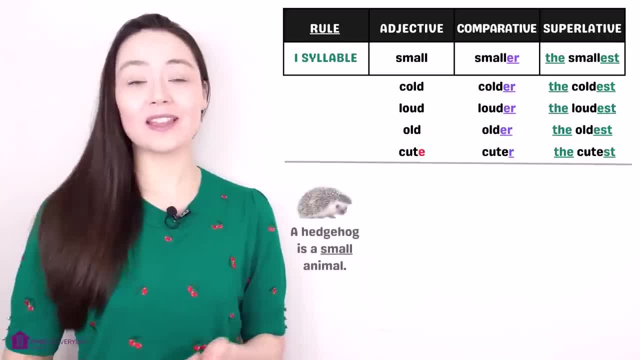 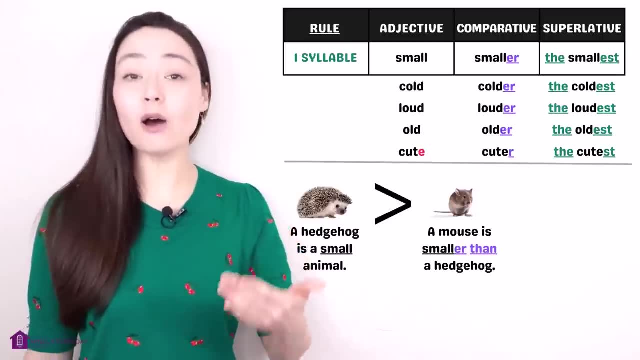 When do we use a superlative? A hedgehog is a small animal. A mouse is smaller than a hedgehog. You can see, we use a comparative to compare two things. Okay, I want you to remember this: Comparatives compare. 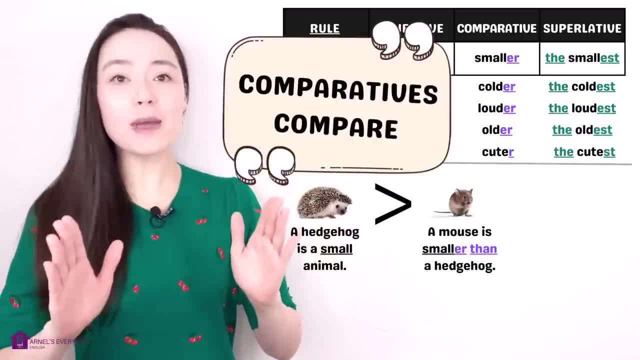 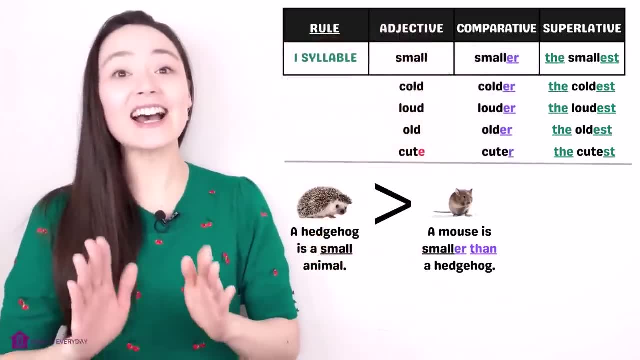 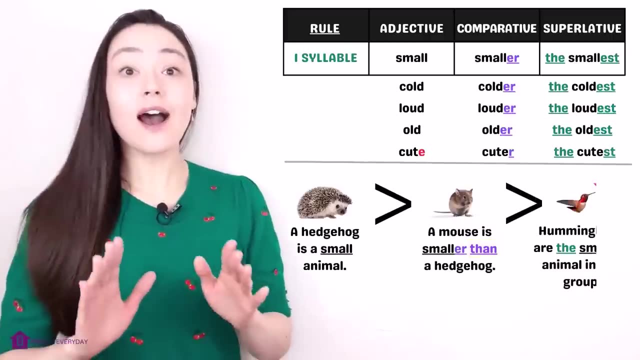 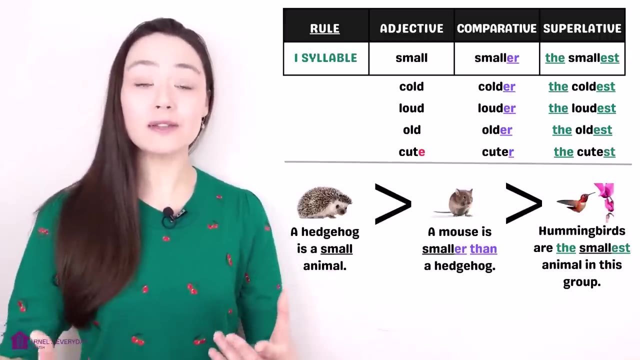 Comparatives compare. You can see comparatives are in the middle of the chart. Why? Because comparatives compare, And I add than Not then, and not that Hummingbirds are the smallest animal in this group. You can see the superlative gives you the most extreme. 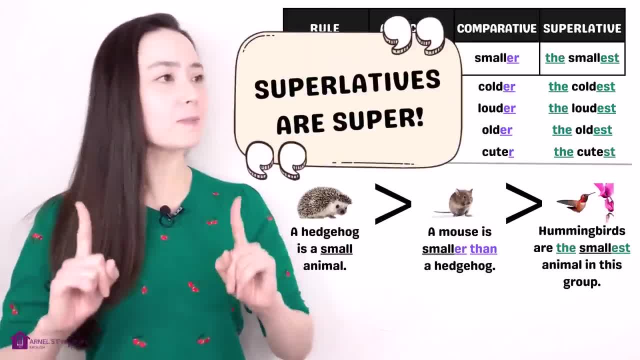 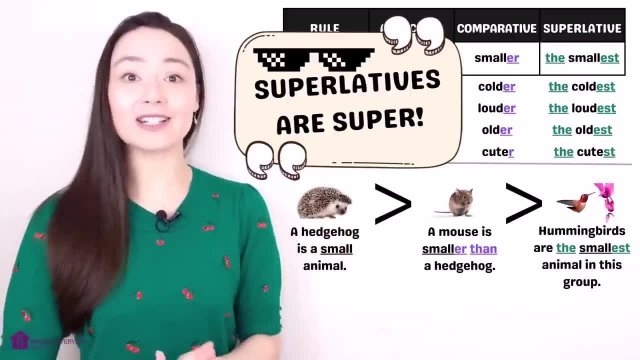 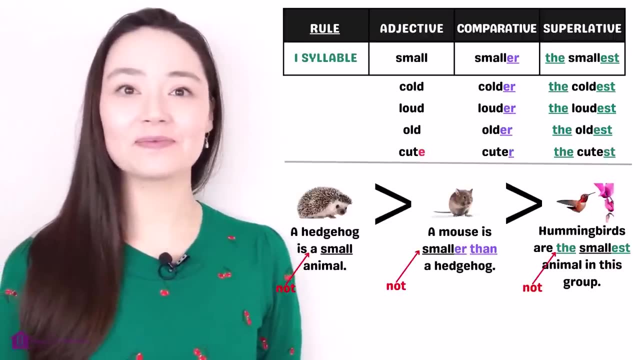 Think about it like this: Superlatives are super. Superlatives are super. They're like the boss adjective. How can I make these sentences negative? I add: not Tuesday was cold. Wednesday was colder than Tuesday. Comparatives compare. 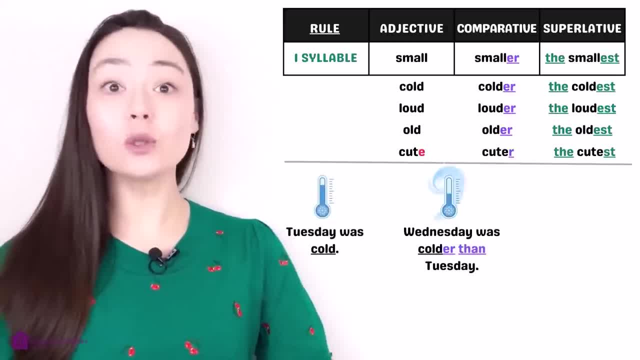 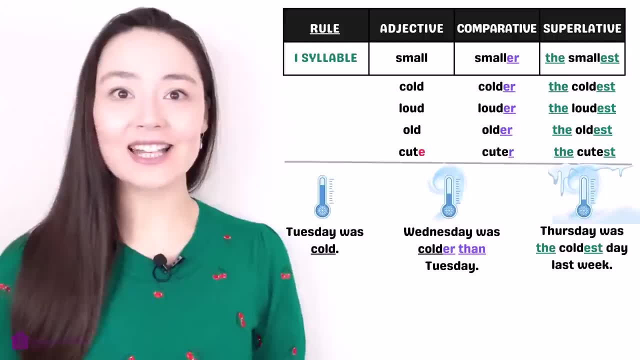 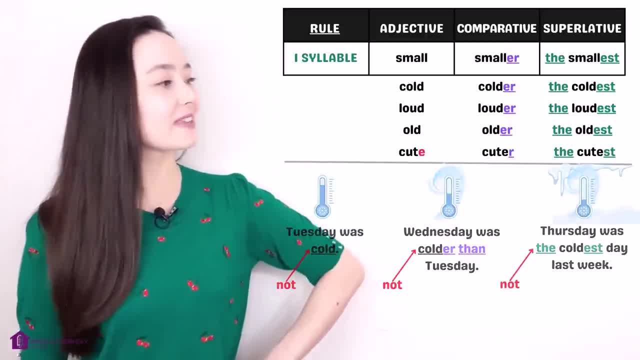 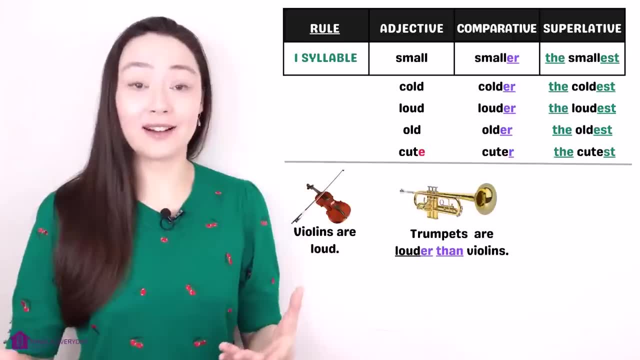 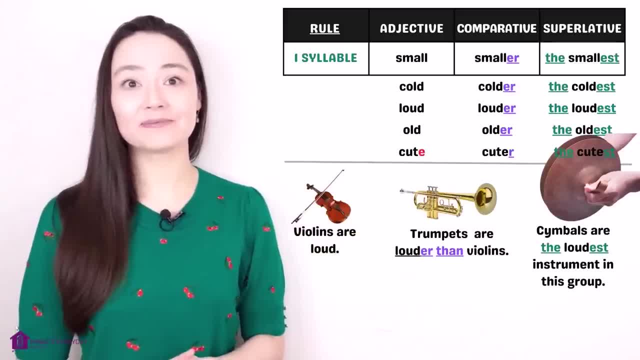 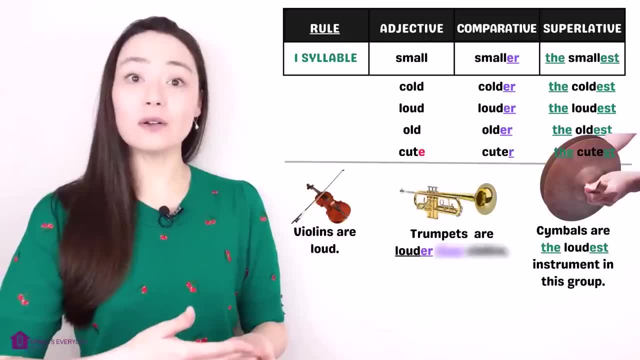 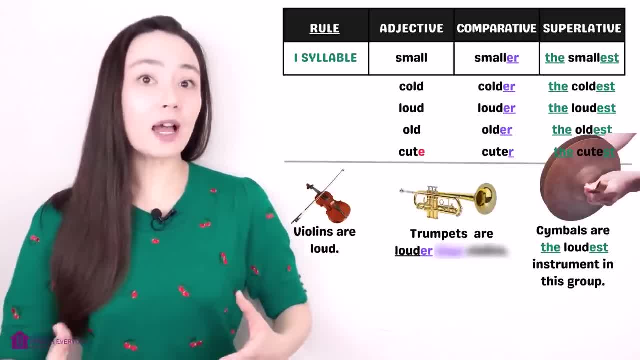 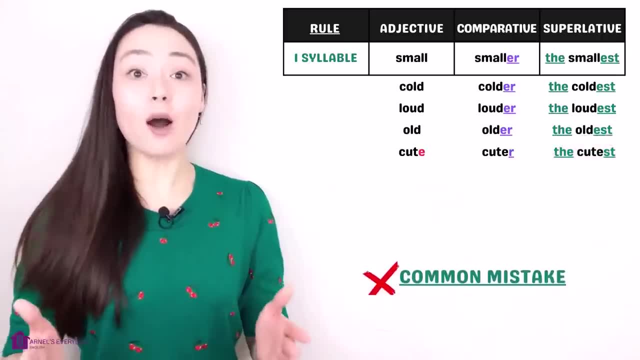 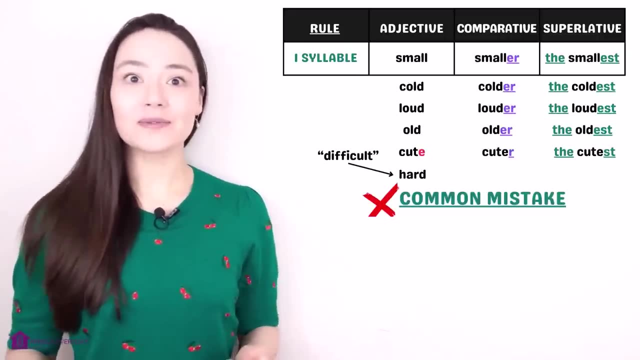 I'm comparing trumpets to violins. so many times you'll see a comparative without them. if it's obvious, Let's look at a common mistake. I'm going to choose the adjective hard. Hard meaning difficult, Hard, harder, the hardest. 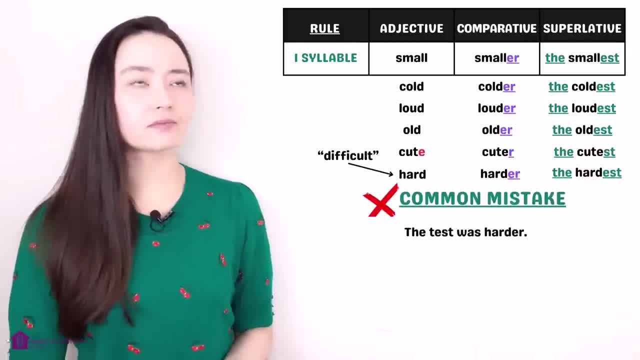 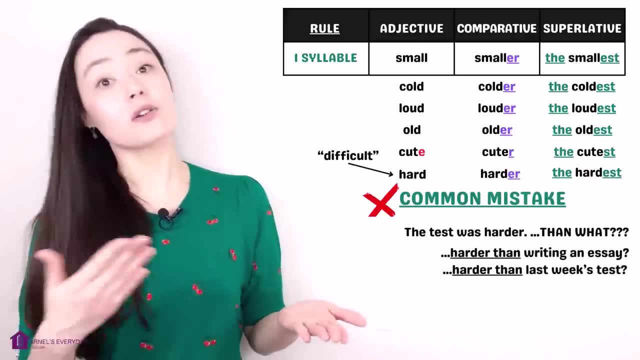 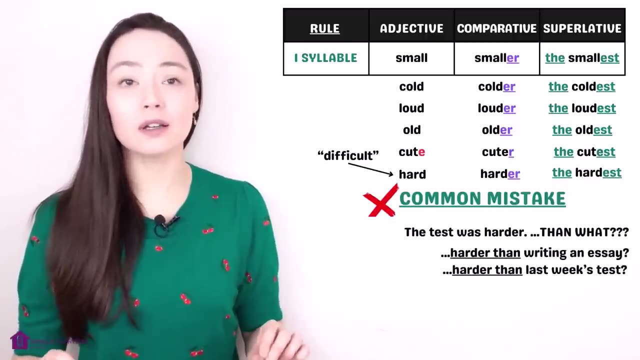 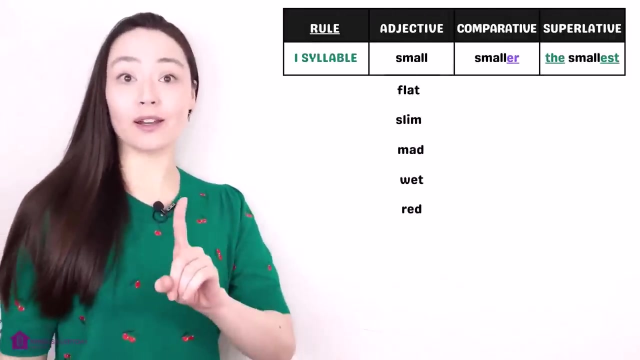 The test was harder. Harder than what? Harder than writing an essay. Harder than last week's test. If you're not comparing two things, don't use a comparative. The test was hard. Here are a few more adjectives with one syllable. Let me give. 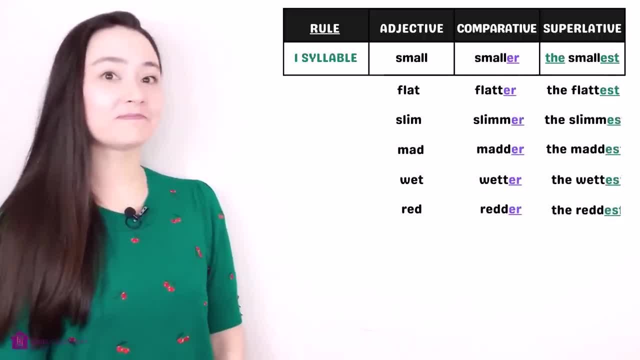 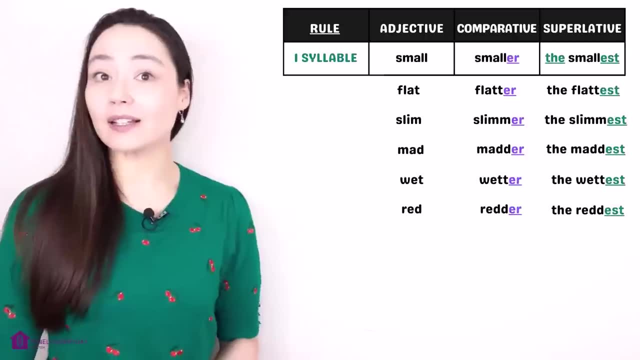 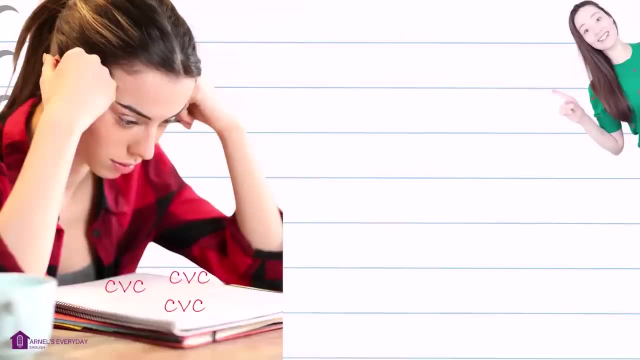 you the comparative and superlative forms? Do you notice anything different about these adjectives? Look at the spelling: CVC, CVC, CVC, What, What do you mean? CVC C consonant V. vowel C consonant. 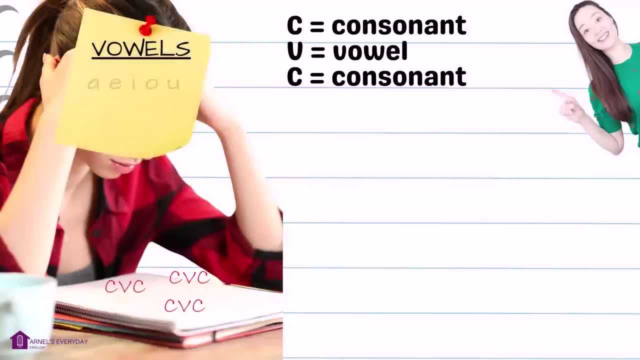 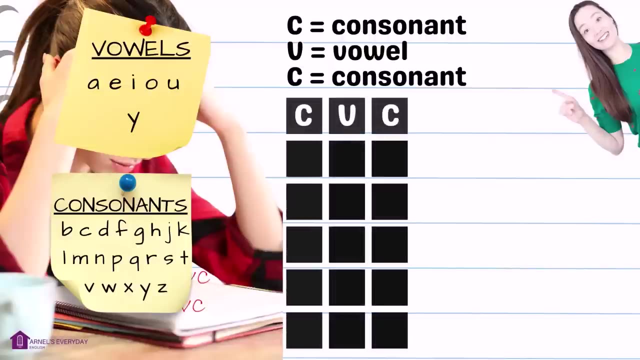 Mini reminder: Vowels in English are A, E, I, O, U. Consonants are all the other letters. Yes, sometimes Y is considered a vowel. If your one syllable adjective has a CVC ending, you double the last consonant, You. 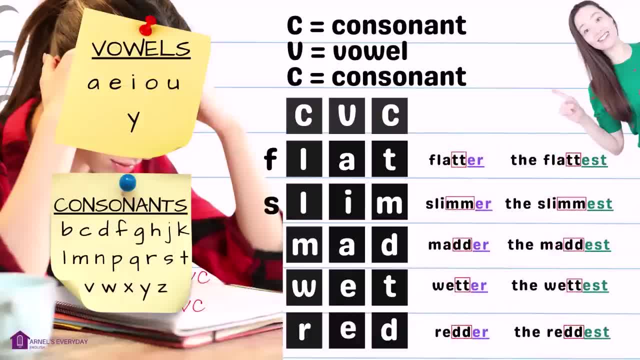 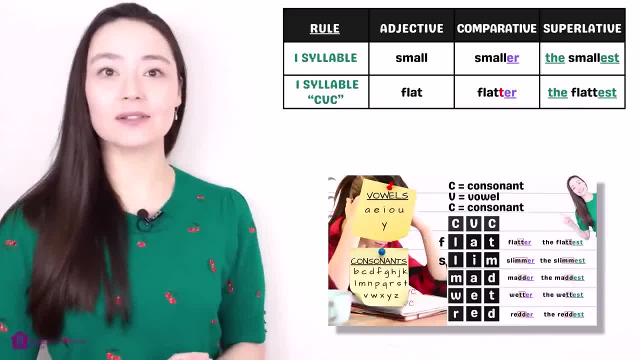 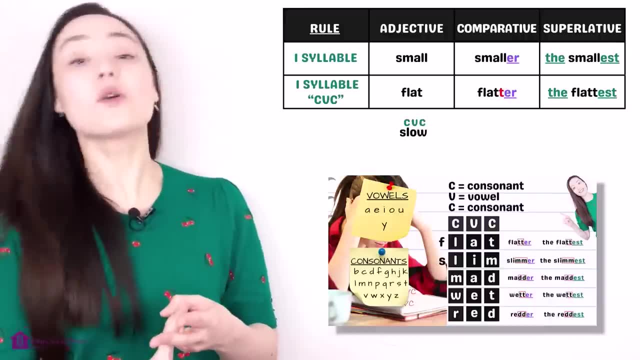 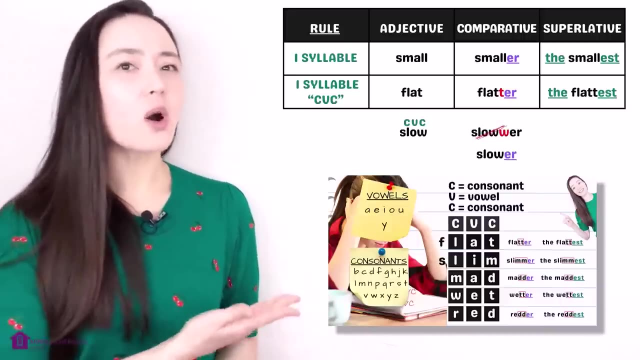 can see that in the spelling. Let's look at an exception, because there are always exceptions: Slow. Slow has one syllable Check. Slow ends with a vowel and consonant Check. But we don't spell it like this. We don't spell it slower, We. 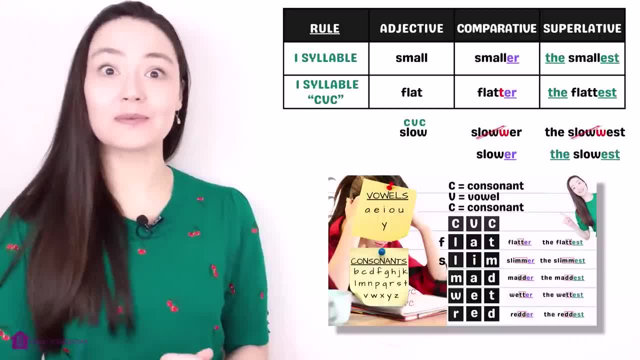 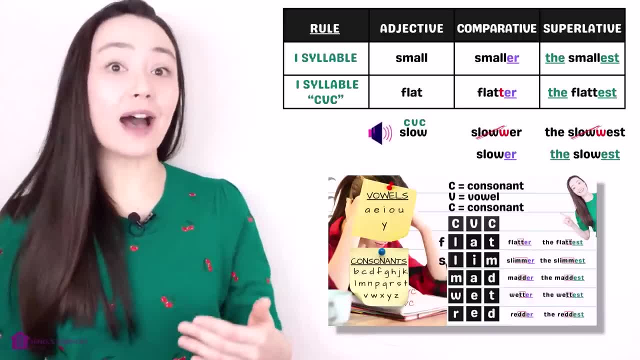 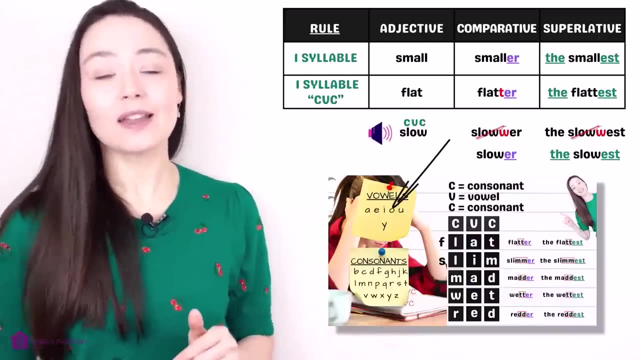 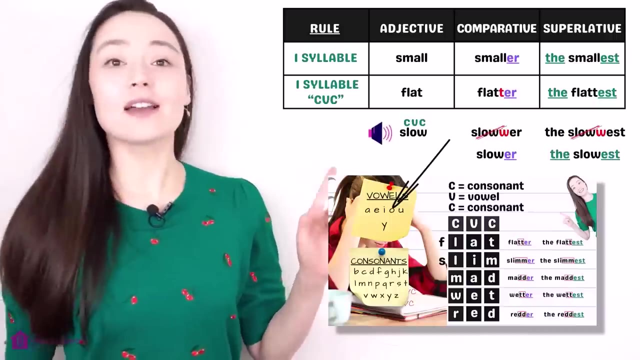 don't spell it slowest with the double W. Why? Well, because think about the sound Slow, It ends with a vowel. sound Slow, Oh, Oh, Oh is a vowel. So in this case, here it's not so much about the spelling, it's the sound. The good news is the spelling. 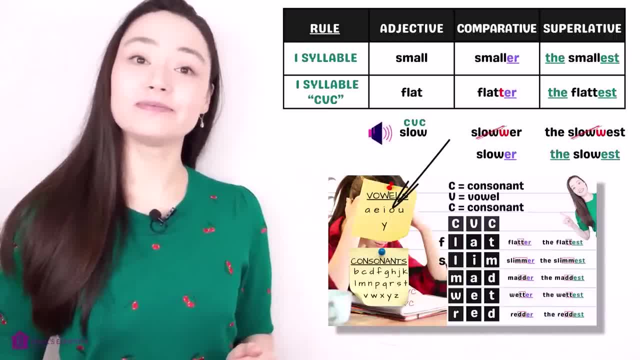 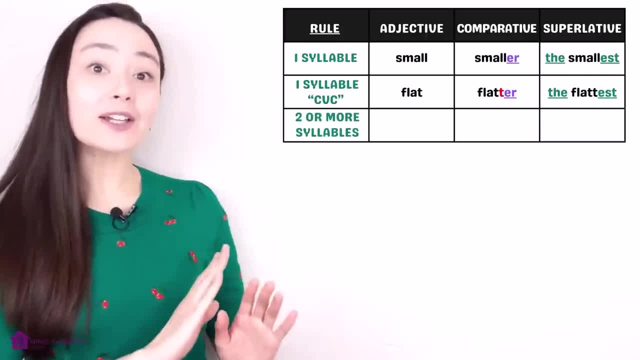 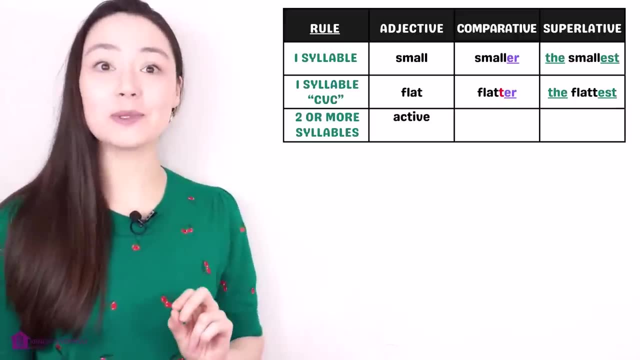 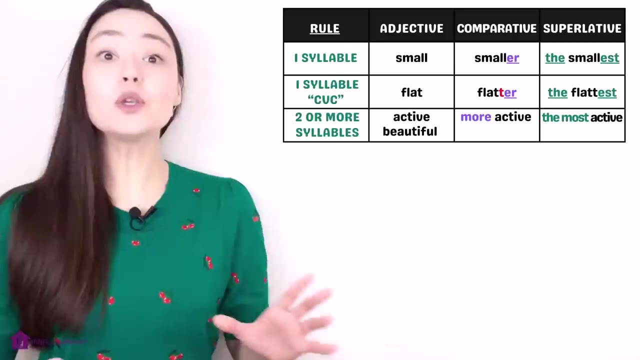 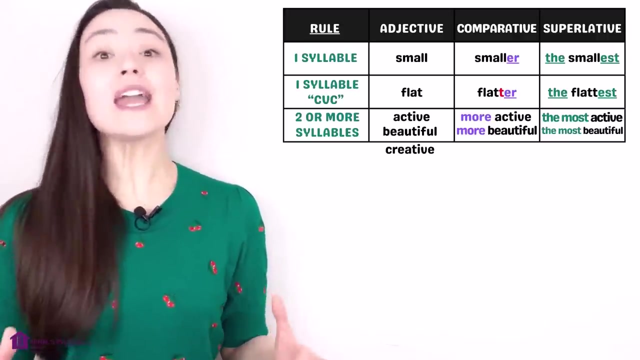 doesn't matter when you're speaking, Let's keep going. You can see, I'll continuously add to my chart Adjectives with two or more syllables Active, Active, Two syllables Active, More active, The most active. Beautiful, More beautiful, The most beautiful. Creative, More creative, The. 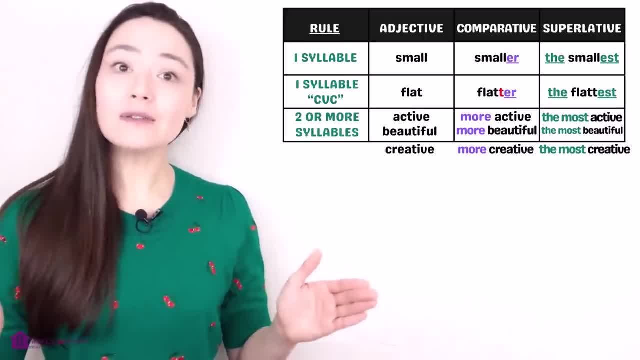 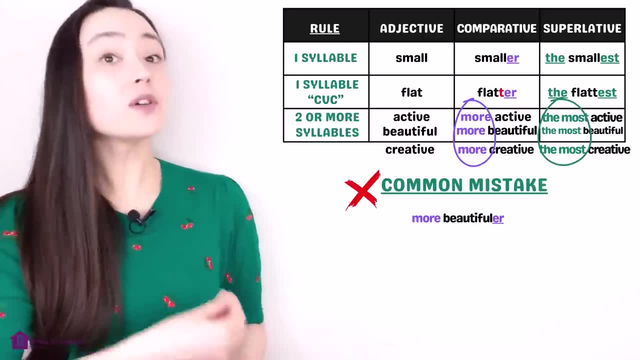 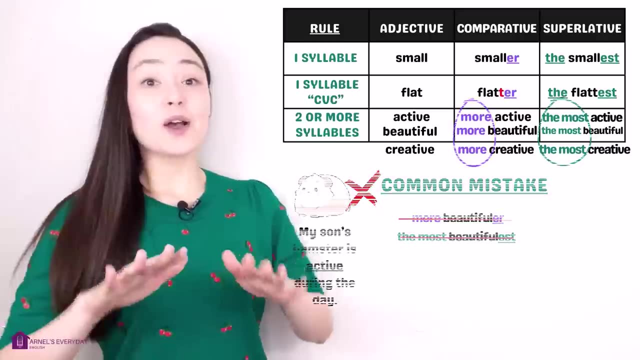 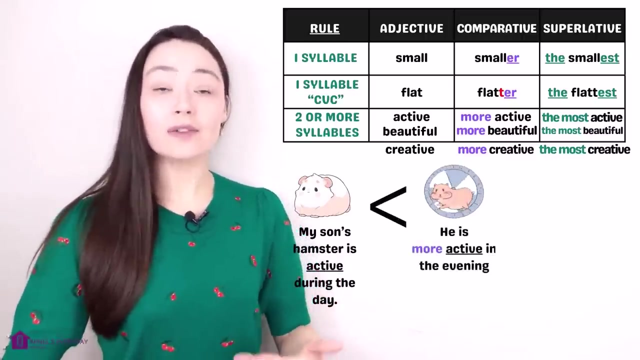 most creative With long adjectives, add more and the most Common mistakes: More beautiful-er, The most beautiful-est. No, My son's hamster is active during the day. He is more active in the evening. I could say he is more active in the. 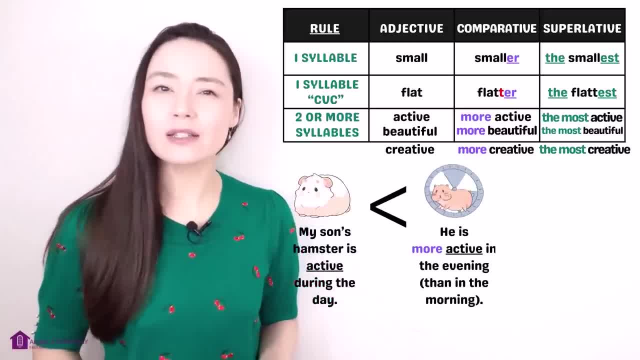 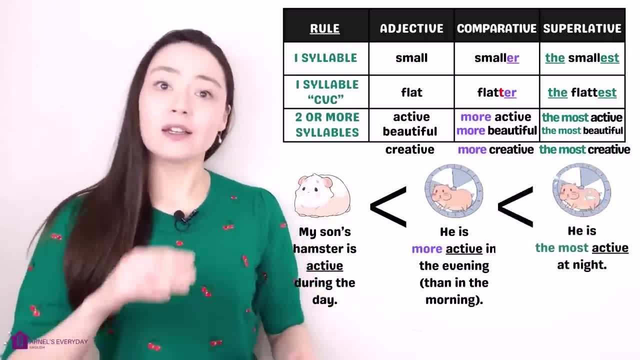 evening than in the morning. but that's not necessary because it's already clear. My son's hamster is the most active, active At night. Squeak, squeak, squeak, squeak, squeak. I can hear it all night. 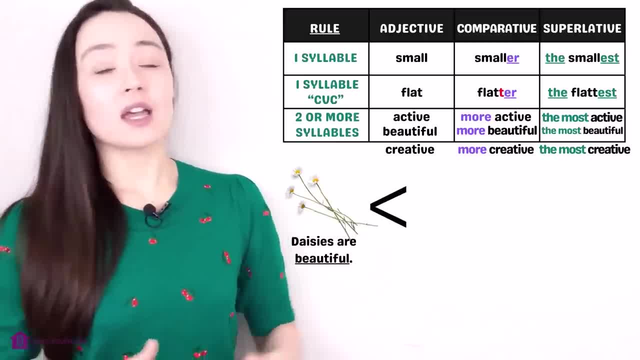 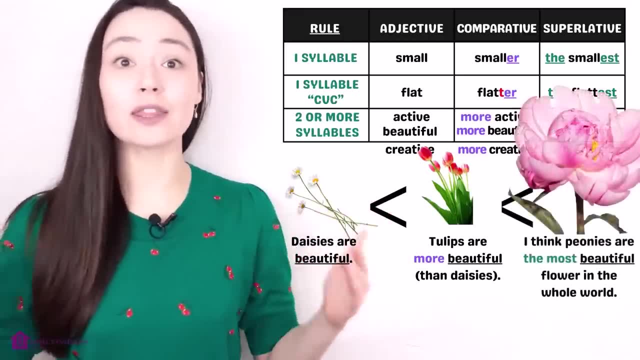 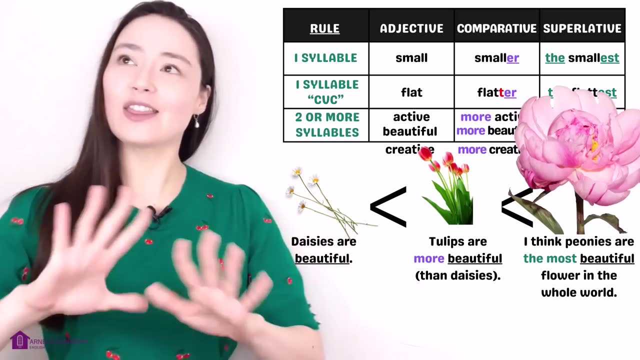 Daisies are beautiful. Tulips are more beautiful than daisies. I think peonies are the most beautiful flower in the whole world, And when you use a superlative, it's important that you do this with your hands. The most beautiful, The most expensive: Kylie is. 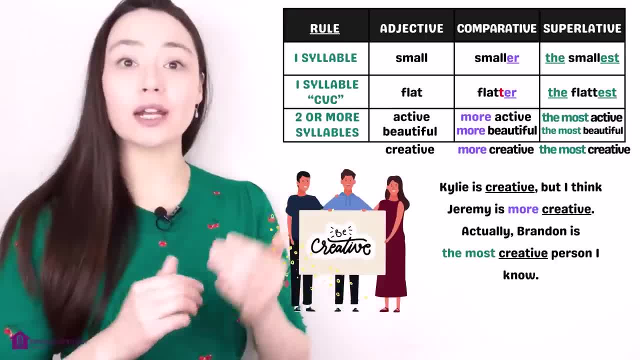 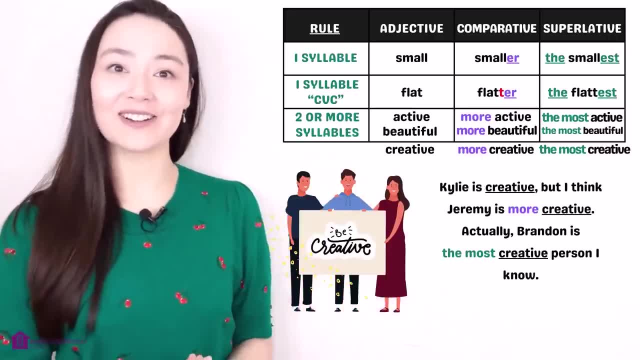 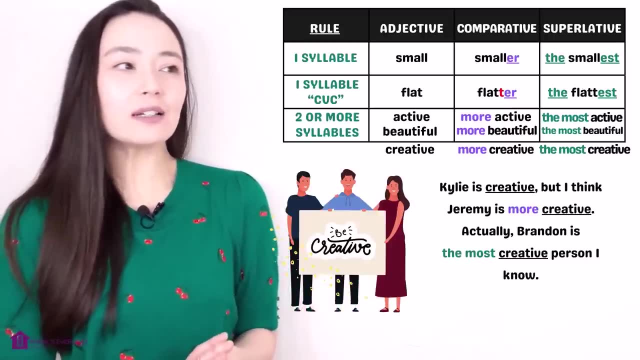 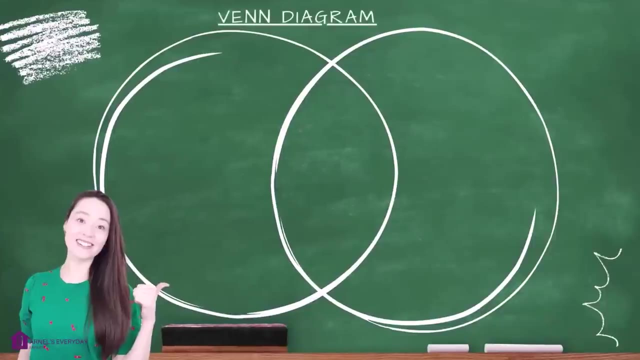 creative, Fortunately. So I said Jeremy is more creative, but I think Jeremy is more creative. Actually, Brandon is the most creative person I know. Let's look at another exception. Yep, another exception. I think we need a Venn diagram. 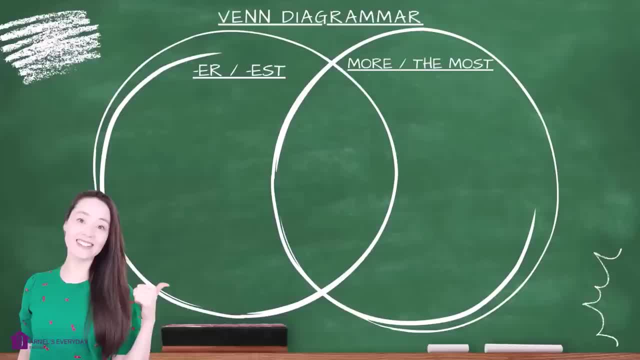 I have my Venn diagram-er here. I have more the most here. We've looked at these two comparative and superlative forms: One syllable cold, colder, the coldest. Two or more syllables frustrated, more frustrated. 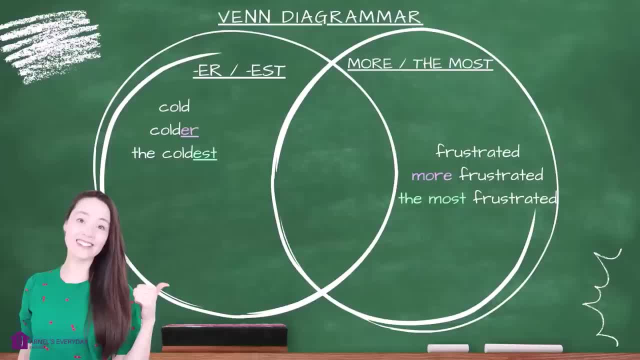 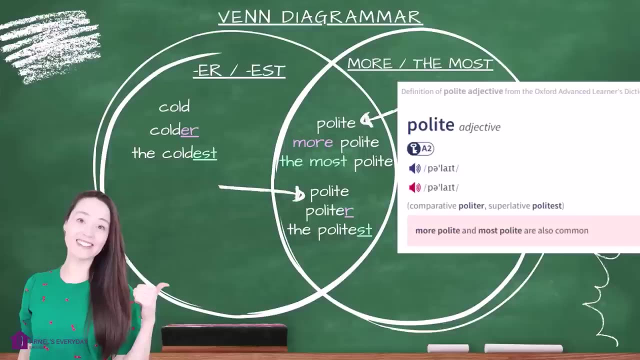 the most frustrated. Some two-syllable adjectives can take two forms: Polite, more polite, the most polite- yep. or polite politer, the politest. Look, I found an example for you here on Oxford Learner's Dictionary. You can see it gives you both options. This is really helpful. 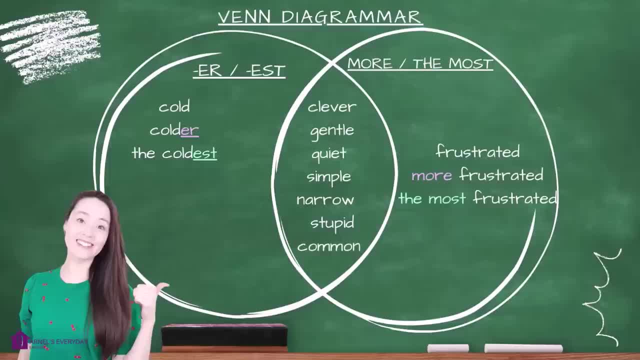 To help you out, here are some two-syllable adjectives that take both forms. I know this can be confusing, but when you hear comparatives and superlatives, just look at what forms are being used, Because not all two-syllable adjectives can take ER or EST. Famous and useless. 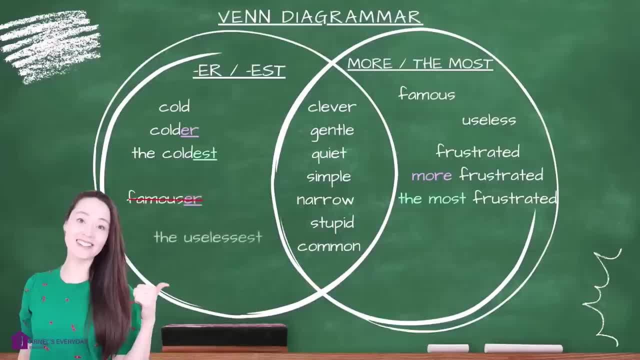 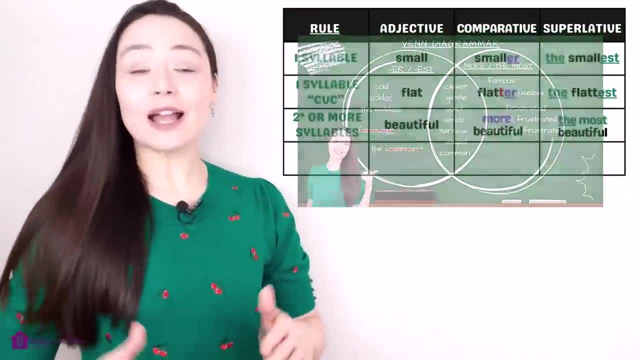 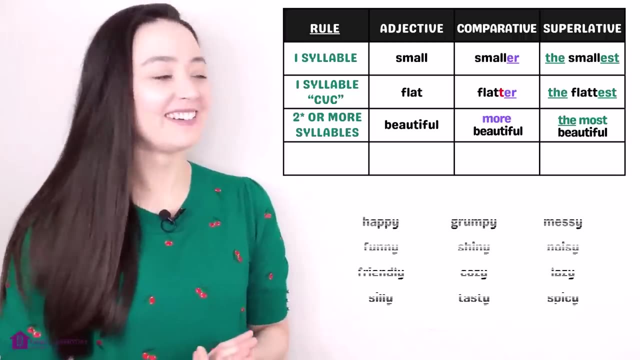 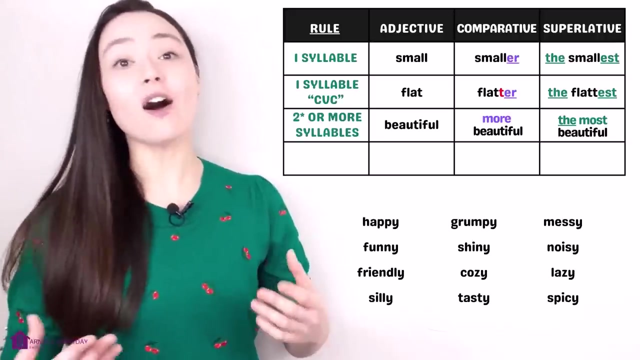 Famouser, No, Uselessest, No. Let's look at some more two-syllable adjectives. Yeah, two-syllable adjectives are a pain. How are these similar? Sure, take a look, They all end in Y. How do we form the comparative and superlative? 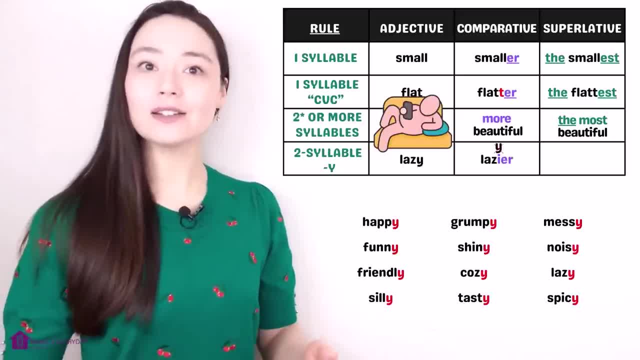 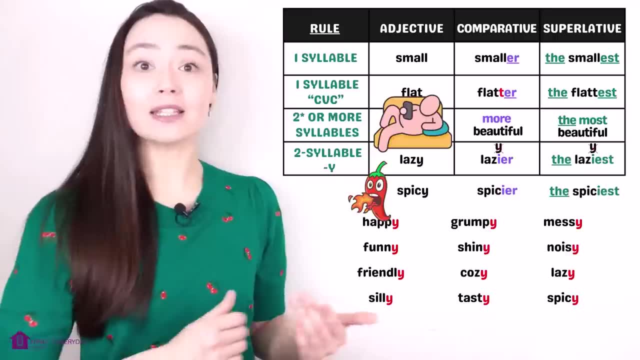 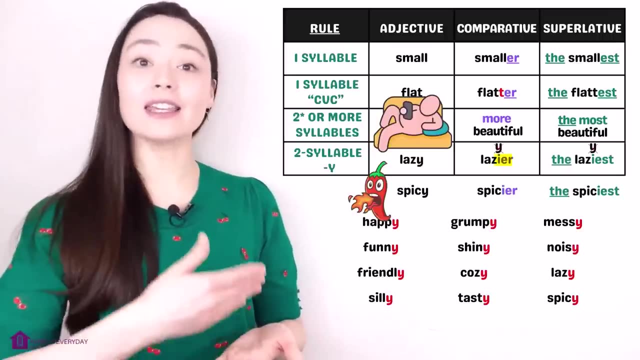 Well, lazy, lazier the laziest, Spicy, spicier the spiciest. If your two-syllable adjective ends with a Y, remove the Y and add I-E-R, R-I-E-S-T. 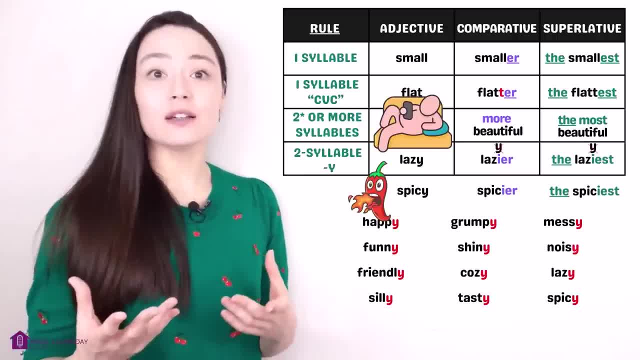 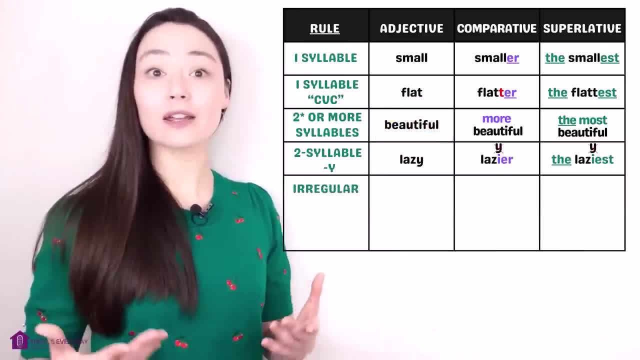 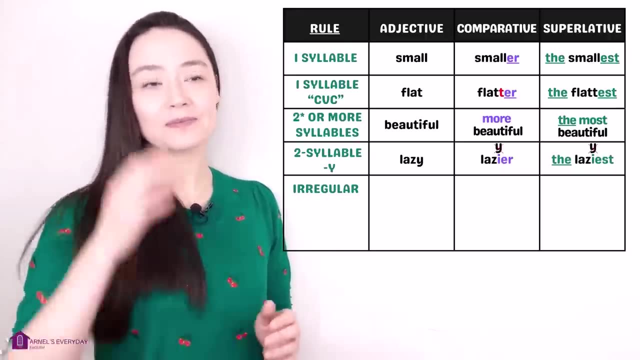 99% of the adjectives you'll see can fit nicely into this chart here. But let's look at a few irregular adjectives, And the good news is there aren't that many. They're pretty easy to memorize. Good, Gooder. 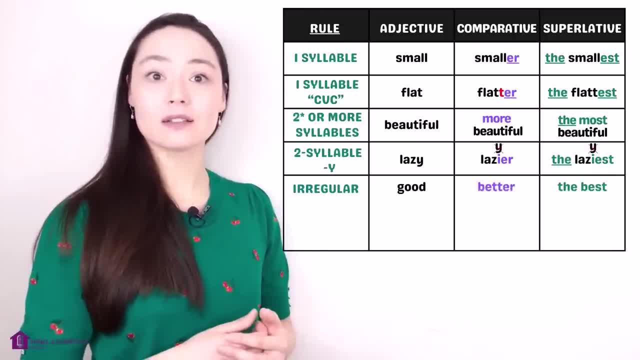 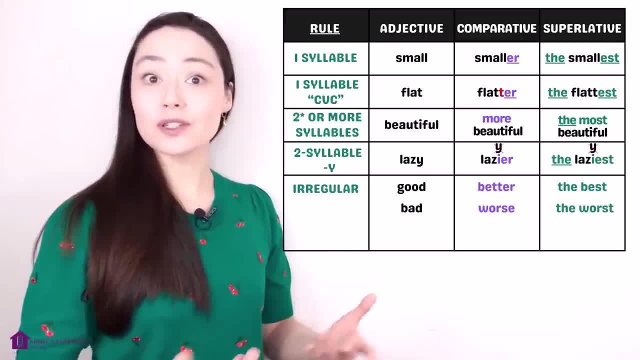 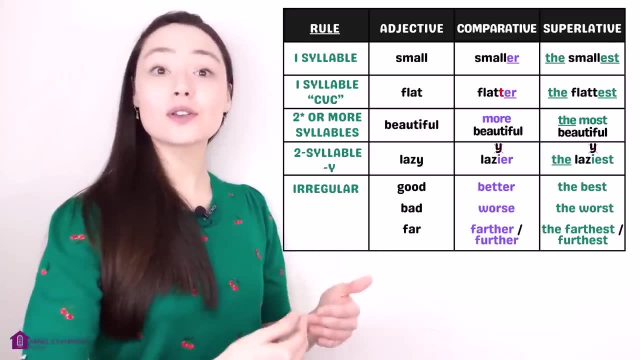 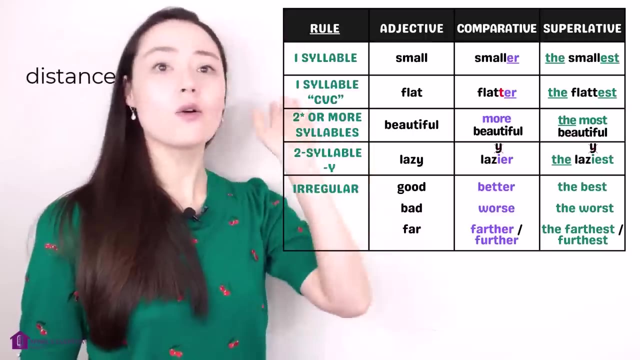 Good, Better, The best, Bad, Badder, Bad, Worse, The worst, Far, Farther, The farthest, Far Further, The furthest. And today I mean far in terms of distance, Far, 100 miles. 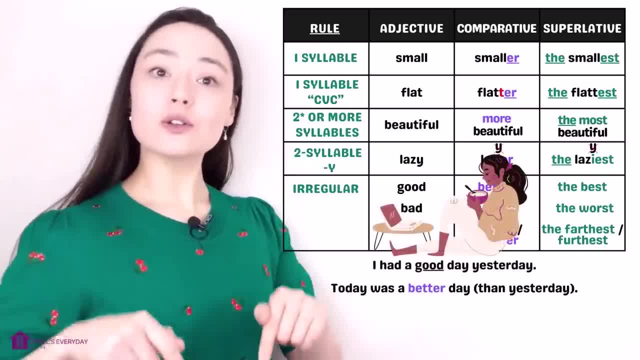 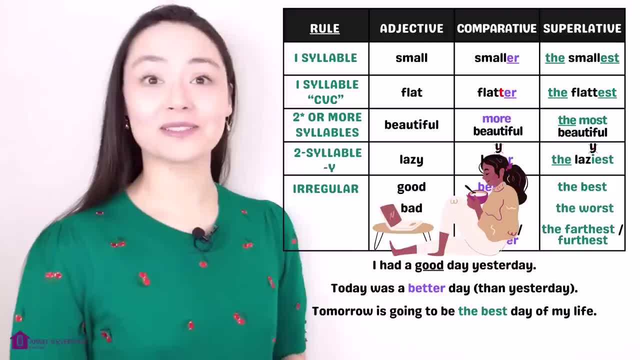 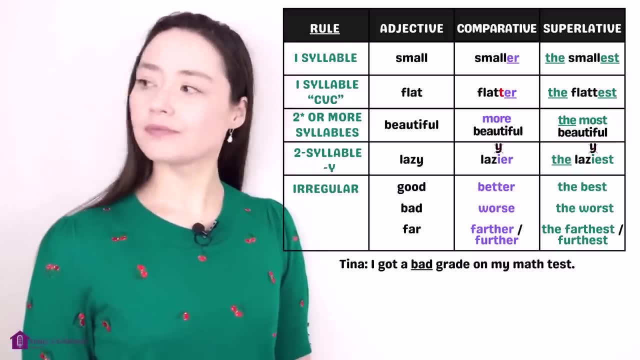 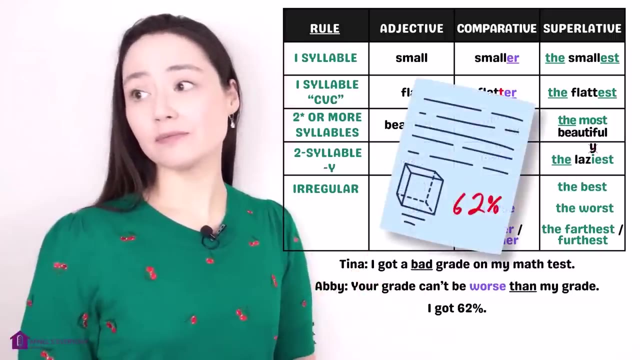 I had a good day yesterday. Today was a better day. Tomorrow is going to be the best day of my life. I got a bad grade on my math test. Your grade can't be worse than my grade. I got 62%. Yeah, you probably have the worst grade in the class. 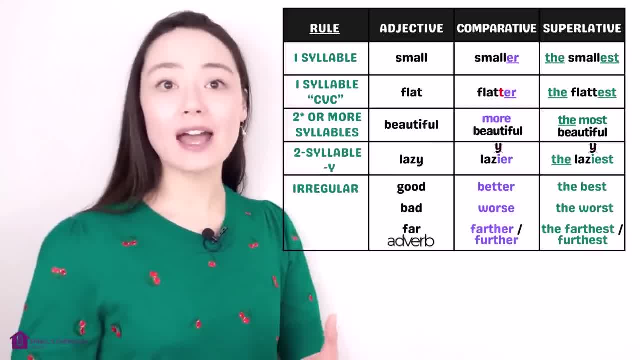 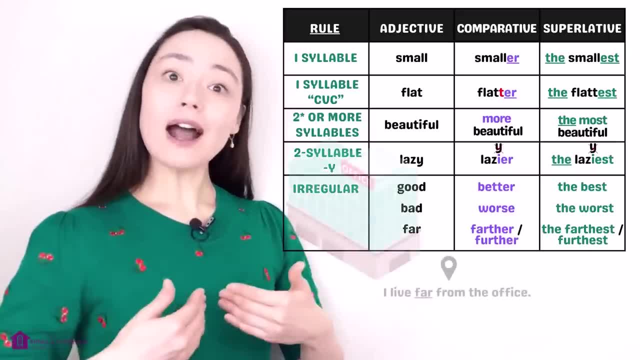 Far is an adjective, but it's often used as an adverb. But the adverb, comparative and superlative forms are the same. That's good. I live far from the office. I live farther from the office than you. 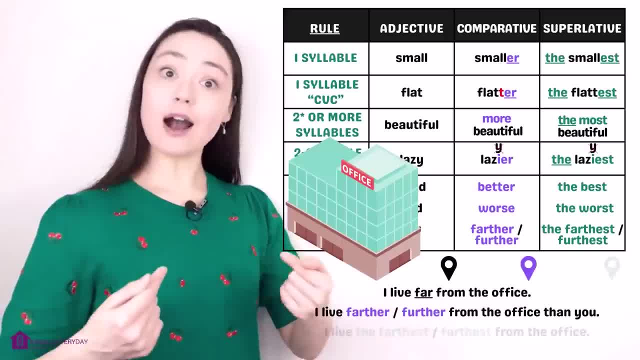 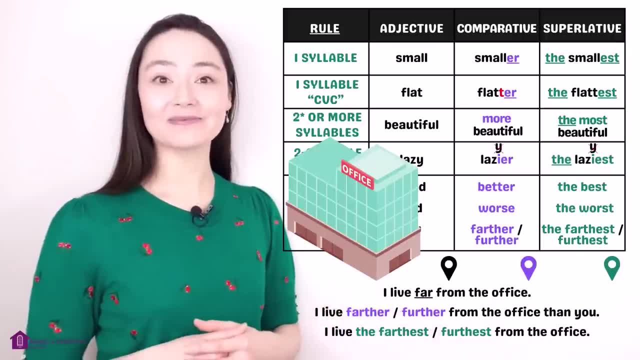 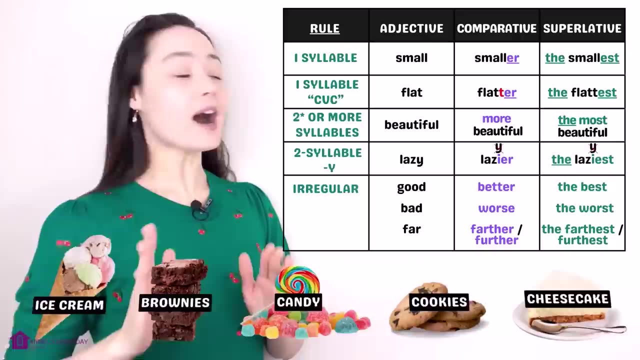 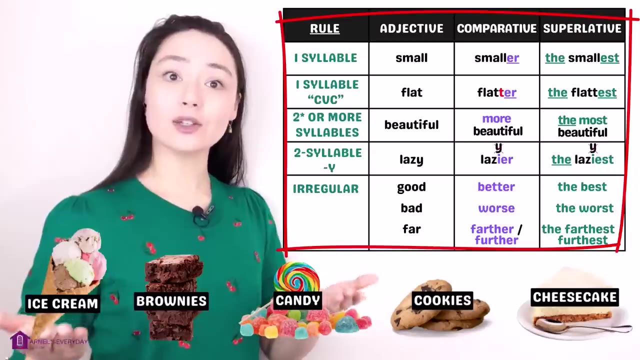 I live further from the office than you. I live the farthest from the office. I live the furthest from the office. Before the test: let's do a little bit more practice. I have five desserts here. Think about all the rules from today. What sentences can you think of? 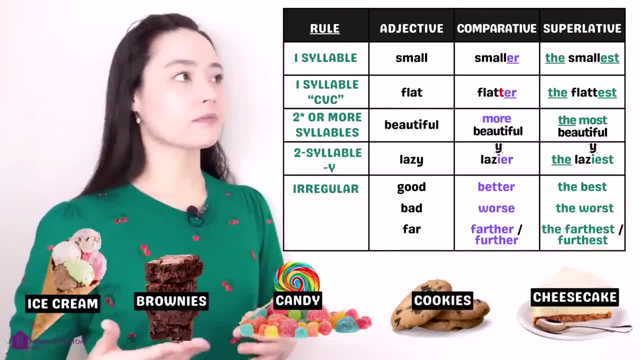 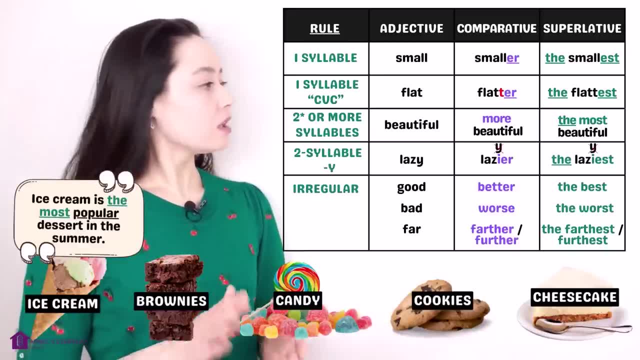 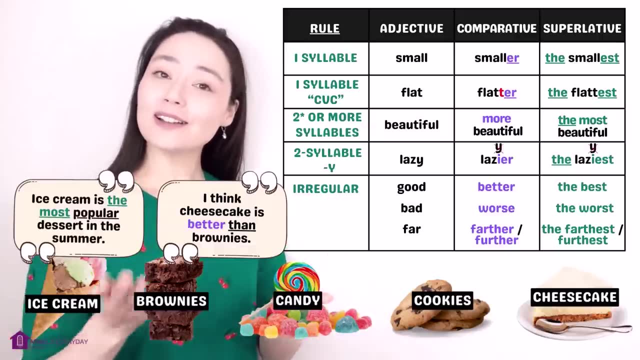 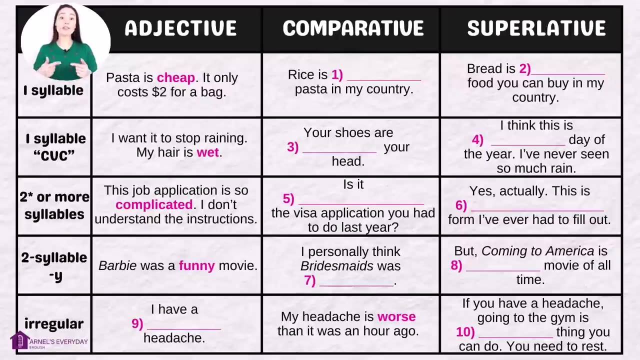 Let me give you two of my examples. Ice cream is the most popular dessert in the summer. I think cheesecake is better than brownies. What examples? can you think of Test time? Remember to think about the spelling of the adjectives.